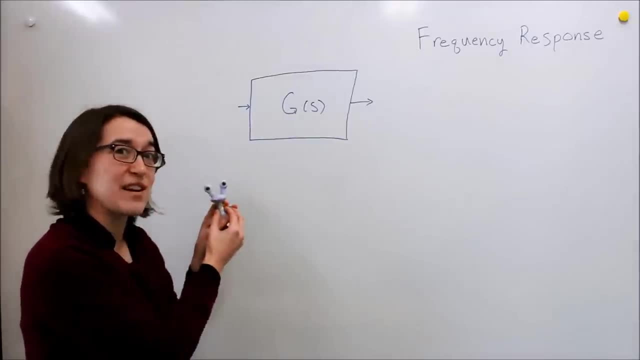 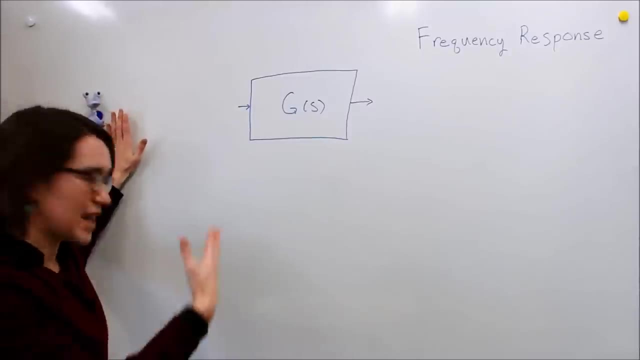 we have. so Valerie, we all know Valerie, she's actually a really great singer And you wouldn't know it, but she's tiny, but she can sing opera. It's really amazing. So say, she can sing a perfect pitch, a perfect frequency, and we're going to put that into. 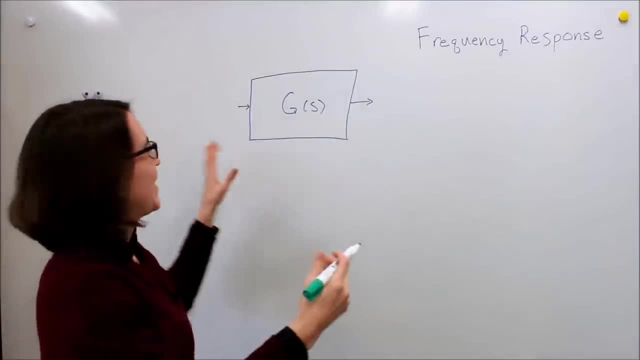 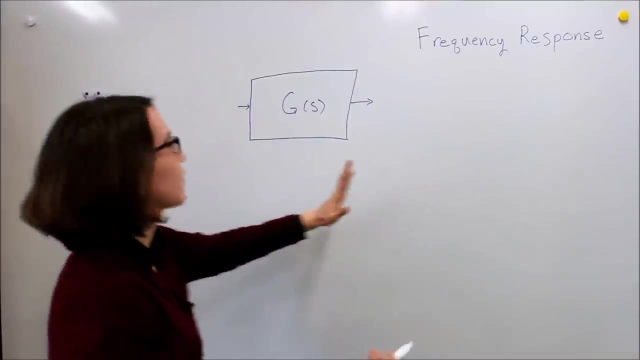 some system, so it's some sound modulation systems, and she's going to put that input. she's going to say, let's sing a frequency into it and we're going to get some sort of signal out. So first let's look at her input signal, so the sound that she's singing. So there's a, we're going. 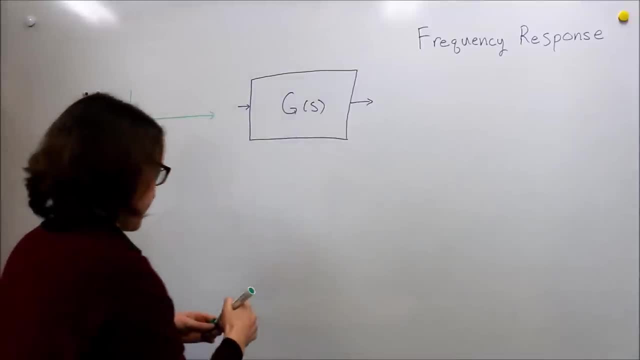 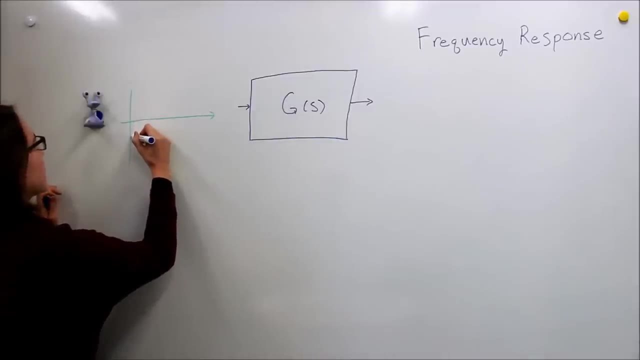 to put it on a time domain. So she's singing some frequency and we're going to say that it maybe starts. we're going to start here and it's some amplitude here. I'm not very good at drawing these sine waves, but 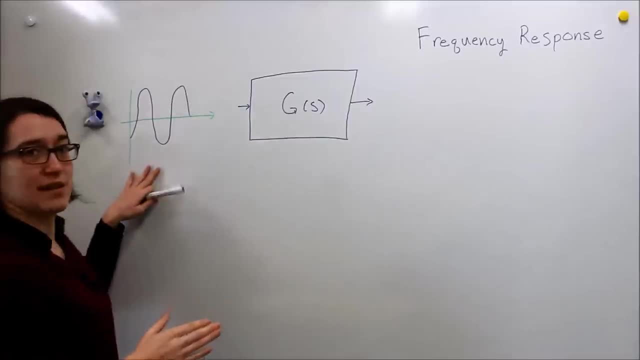 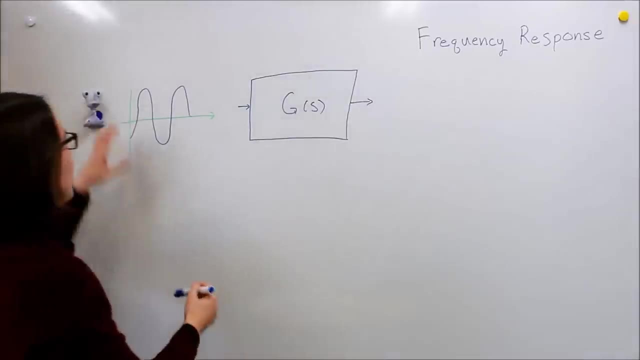 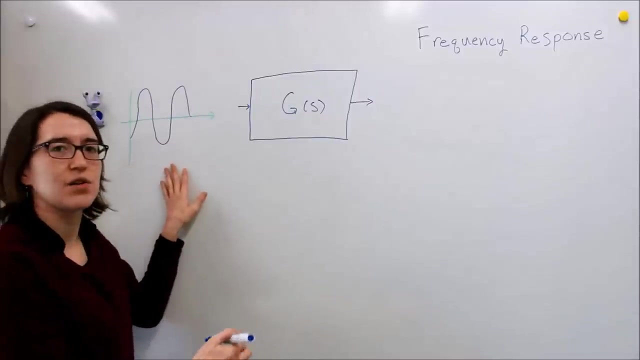 we'll go with it. Okay, so we have this input signal and we're going to use the idea of a phaser. so we're going to look at the magnitude of our system. So we can break this as a sine or a sum of a sine and cosine, but we're going to change it into a magnitude and a phase. 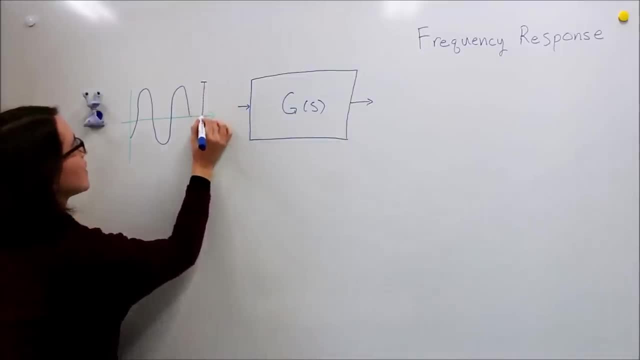 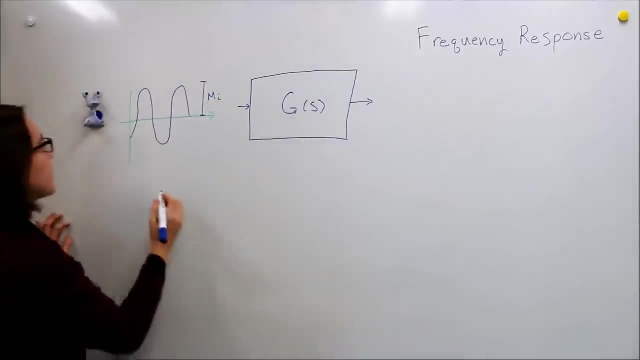 shift. So the magnitude is simply going to be this amplitude from the peak to zero. So that would be. we'd call that M and we're going to call mi for the input, and so this is going to be: mi is our frequency, sorry- is our magnitude. 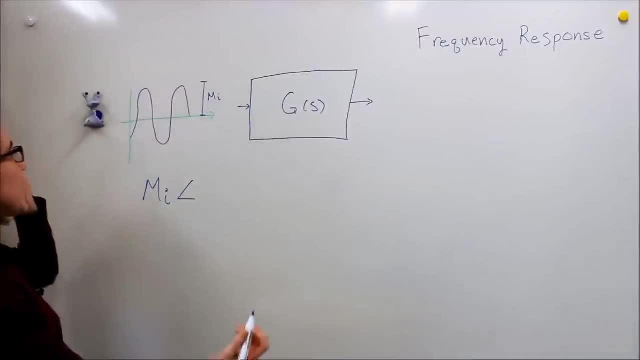 and then in phasor notation you have a magnitude and an angle, And here the angle is going to be so, it's going to be this phase shift. so say we're going to start off, say our starting point is from here, we have some phase shift of that. 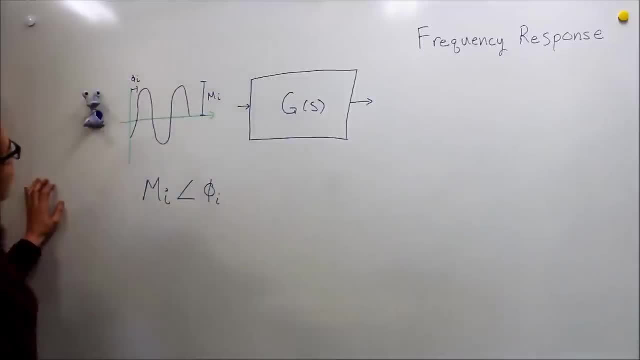 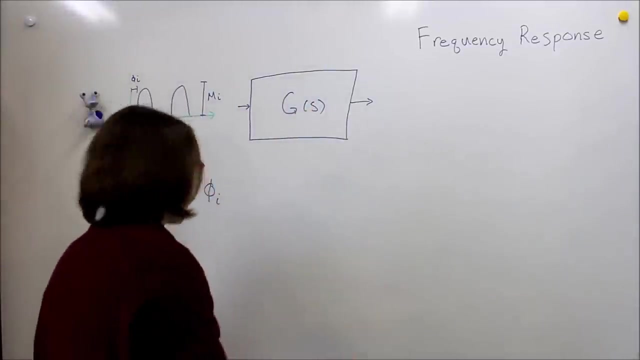 So this is our input. sorry, this is phi i and phi phi phi one of those. so this is our phase shift, our input, and then this is our magnitude. Okay, so we put that into our system and we will get out some system. so say: 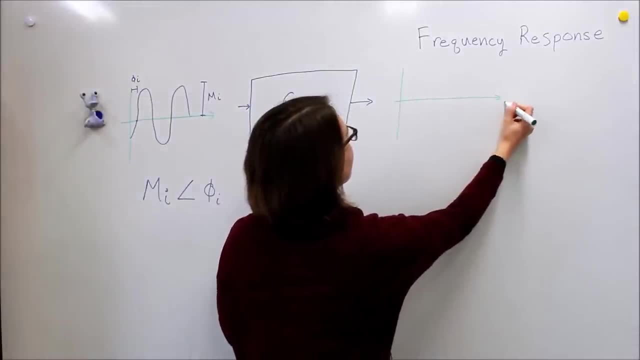 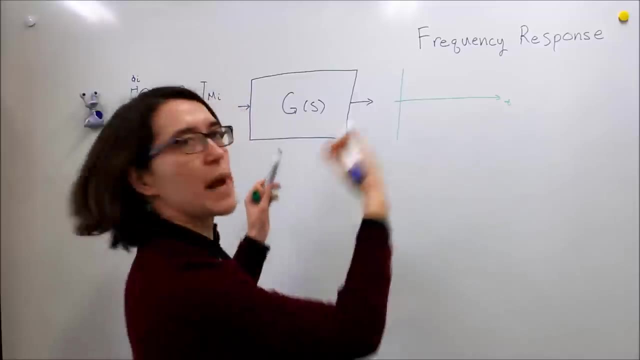 so here's our. I'm going to put on the time domain again. this is time. this is the amplitude of the signal and this time it's going to. this is going to. So here's our. I'm going to put on the time domain again. this is time. 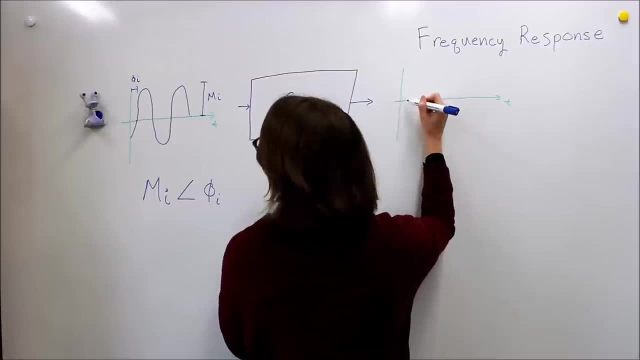 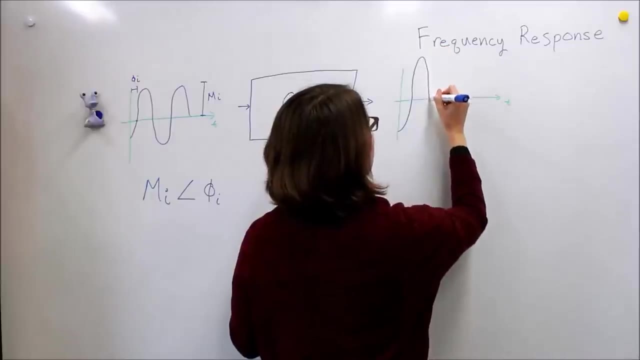 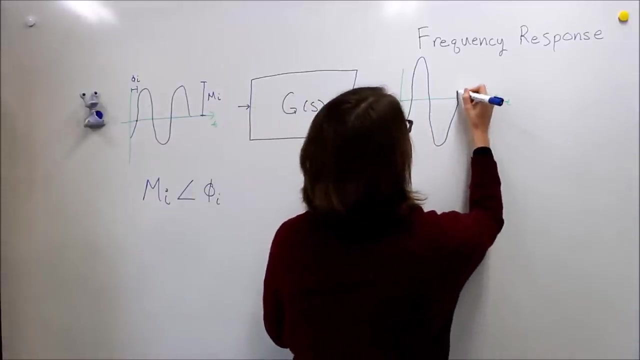 amplify our signal, so we're gonna say it's amplified. I'm not very good at drawing these. okay, let's do one more you can. you can go ahead and use your imagination and pretend it's a nice sine wave, but the point I want to thing I 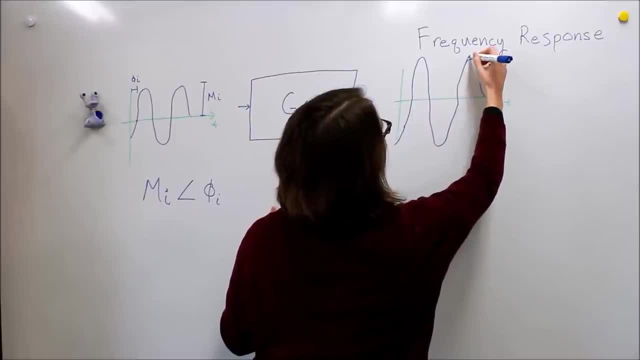 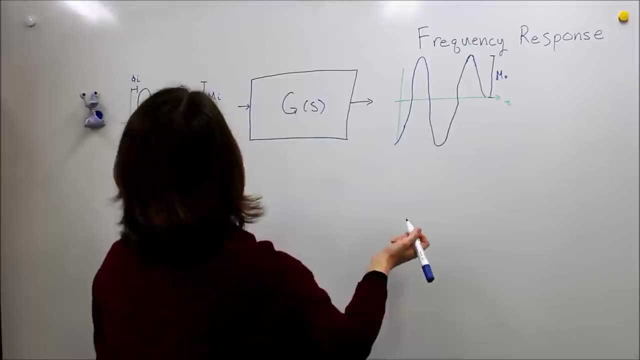 want to show here is that we have- this would be the same amplitude- we have some amplitude out, we're gonna call it M 0 MO output, and then we have some phase shift as well. so here it's a little bit different phase shift. it's changed a. 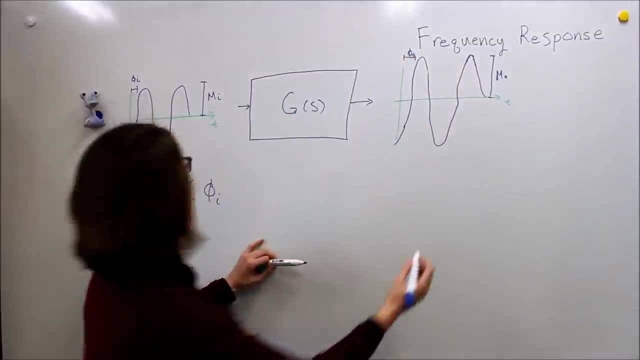 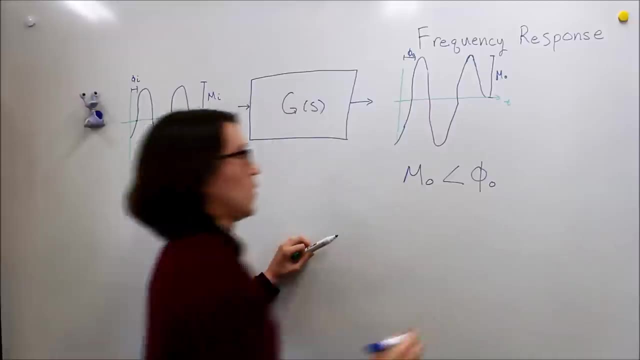 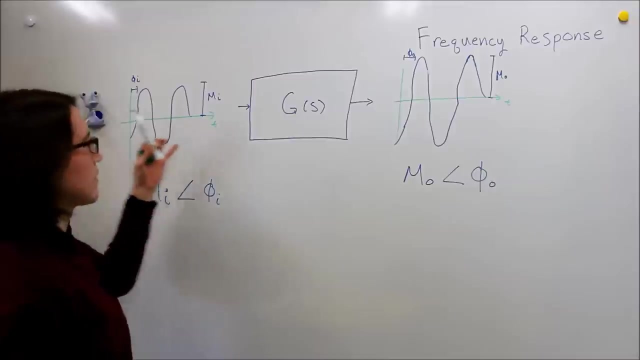 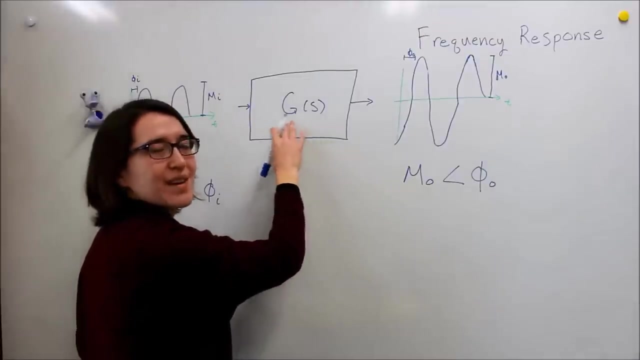 little bit. now we're going to call that V out. so here's M, our signal, here is MO, VO. so this is our input phaser, this is our output phaser and in each of these, when we do just this, just individual frequency, we can model how this system will affect our input versus output. so we can. 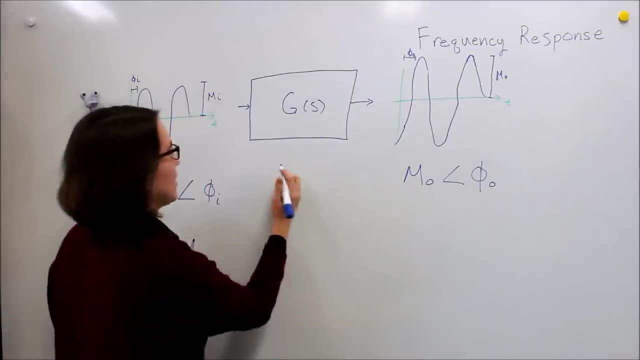 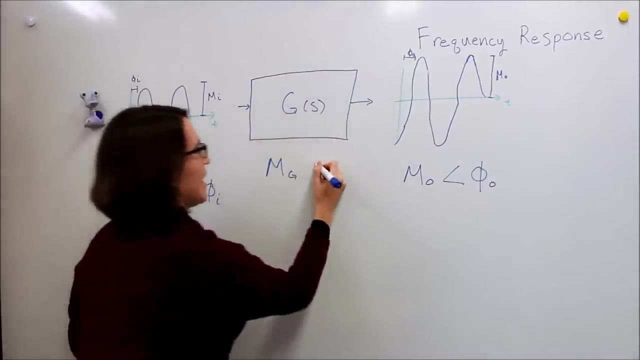 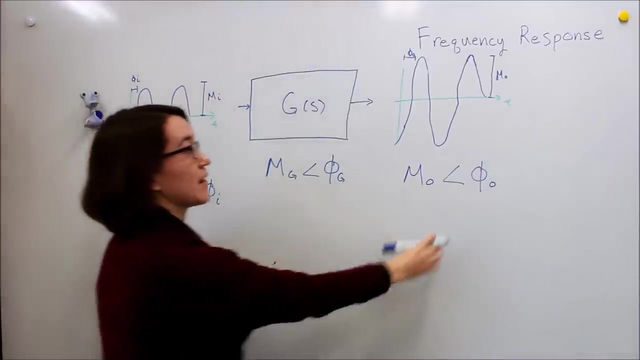 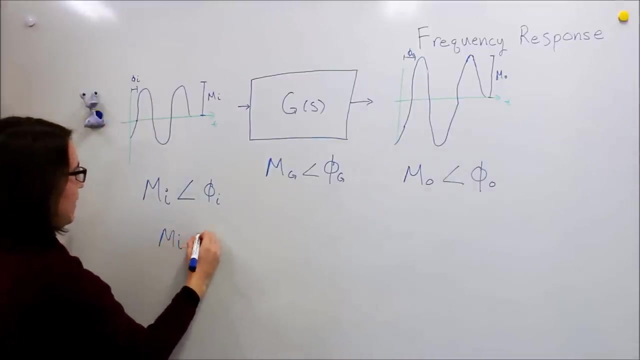 essentially model this only in this situation as a magnitude of this transfer function and a phase shift that it will cause, such that when you multiply these two together you will get this output. so essentially you have this M I and this I, and I'll write it out. so M I VI multiplied by M G. 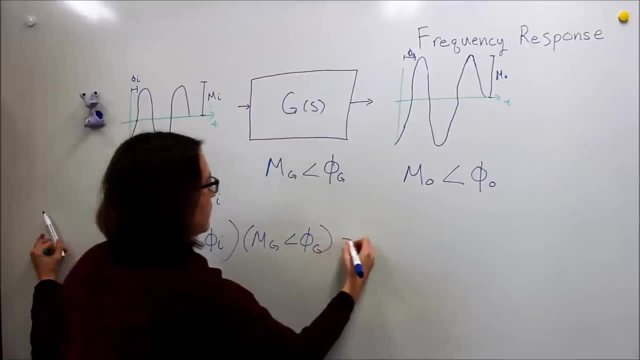 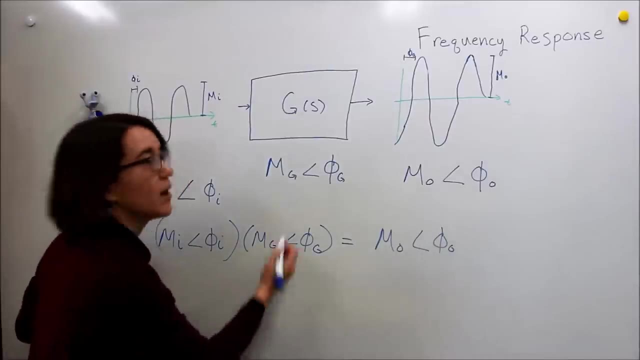 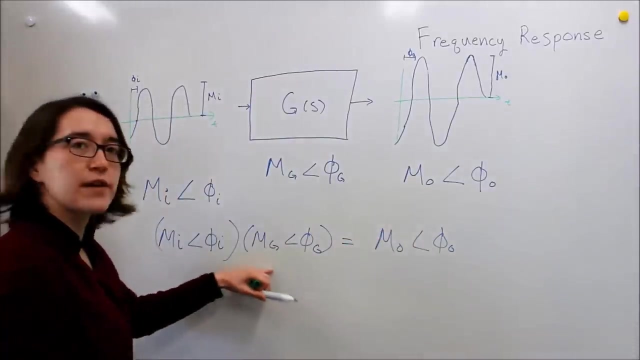 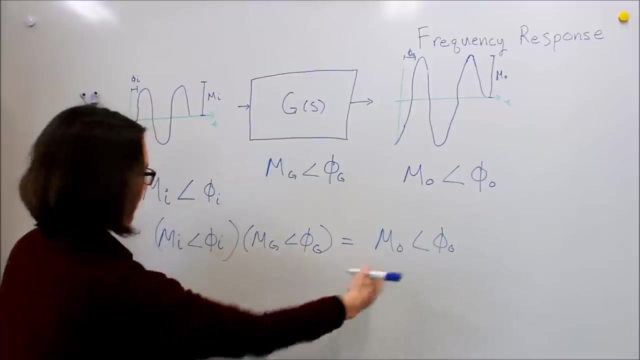 VG is equal to MO VO. so this is essentially our transfer function, but only for an input of frequency and an output frequency. so we call this the frequency response and without going through all of the math, I can tell you that actually. so I'll rewrite this, let's just move it over. 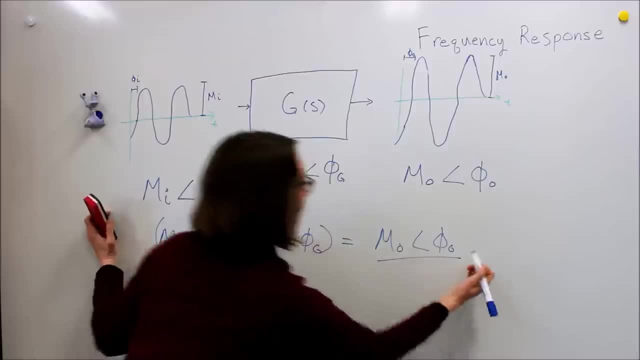 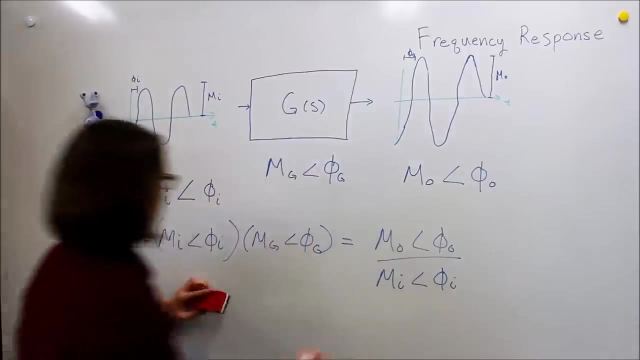 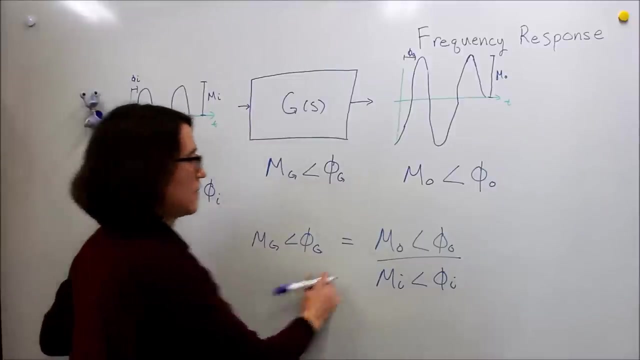 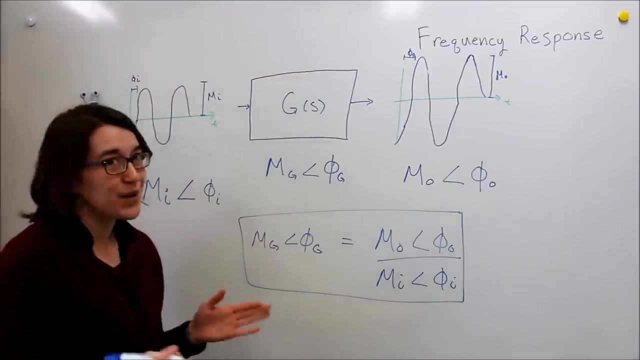 here. so if we want to think about this like frequency response- remember it's the output of the input. so we move this over, we'll get this alright. so we can now get rid of that. essentially, this is our frequency response. so the next question is: how do we find this without going through all of the math? I'm just 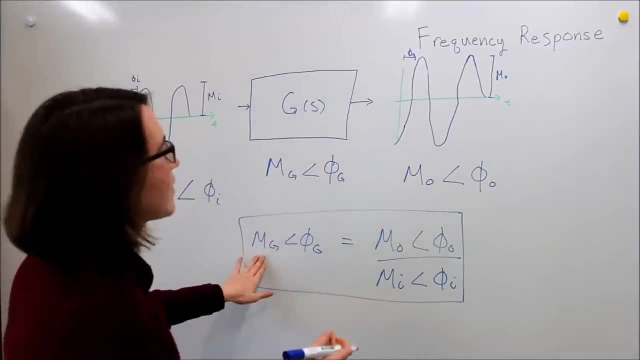 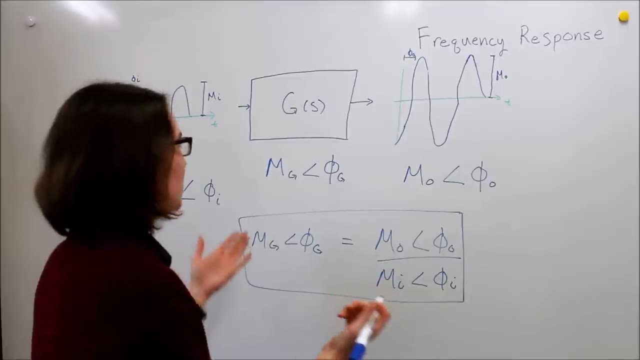 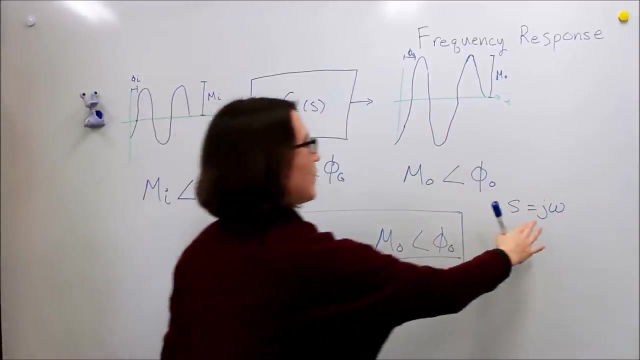 going to tell you the answer. so what we can do is we actually know that we can look at how the system reacts when we put in a frequency signal. so what we do is we make s equal J Omega in this case. so, and if you think about this on the 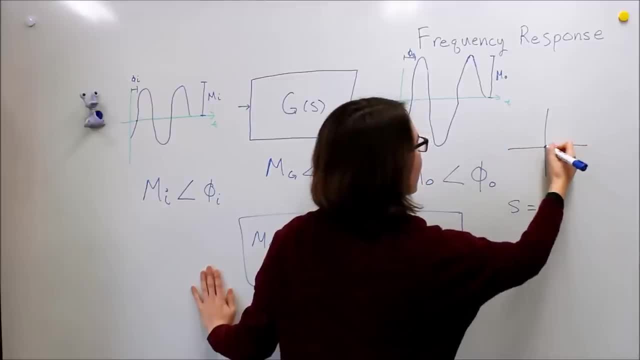 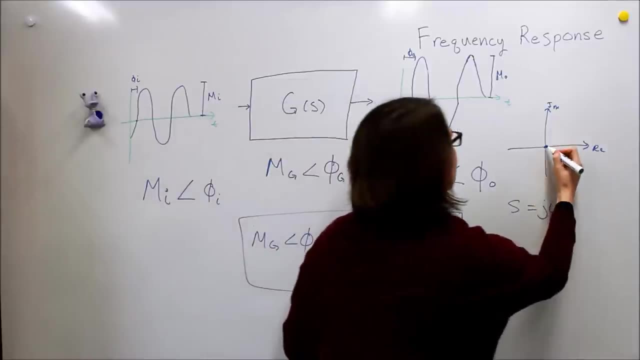 imaginary and real axis that is starting from. so this is real and imaginary, imaginary and real and imaginary. and if you think about this, on the imaginary and real axis, that is starting from. so this is real and imaginary and we are starting from. it's anything essentially, on this, this area, it says on: 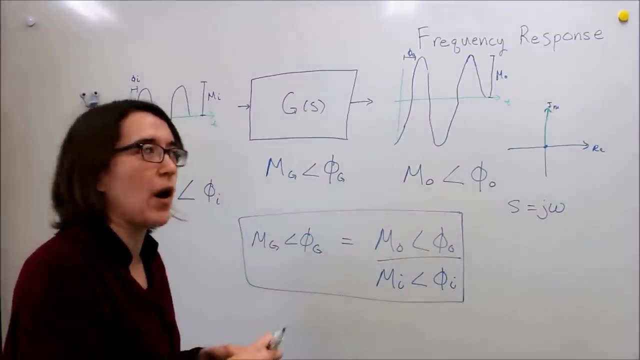 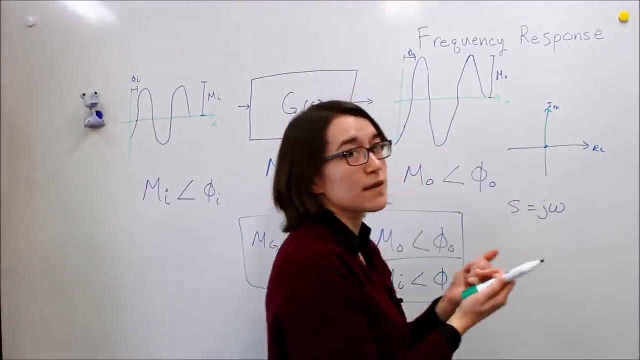 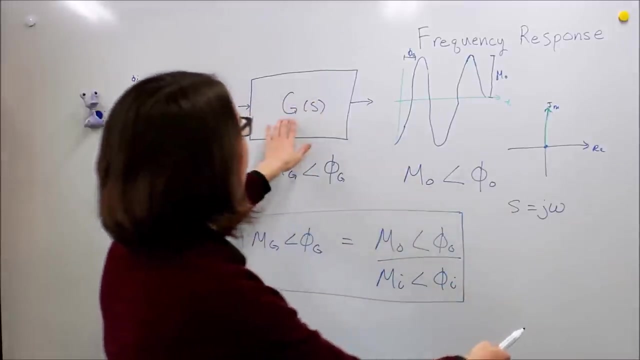 the imaginary axis which, if we remember, that's where our marginally stable occurrences can happen, and we can associate these points with a frequency. so, in short, we can put: if we make s equals J, Omega, and put that into our transfer function here, and it turns out: 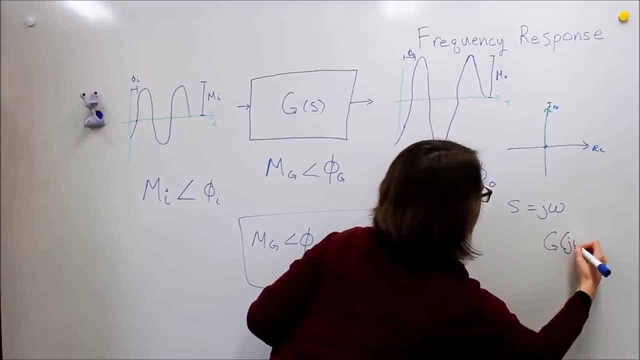 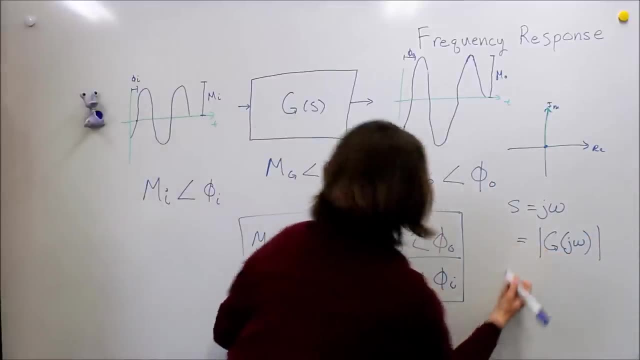 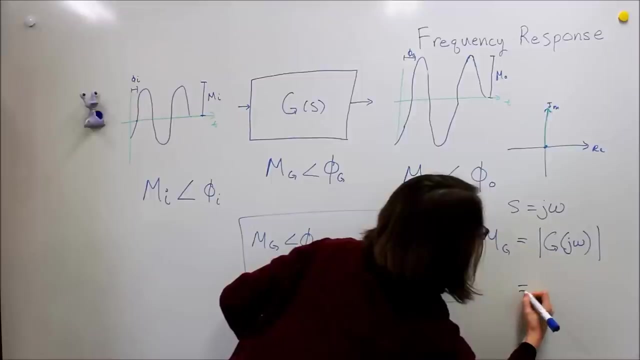 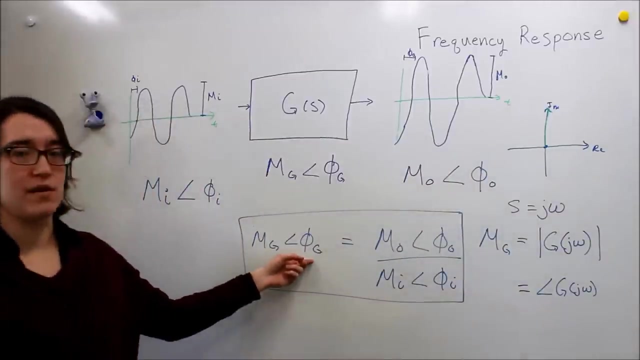 that. so G of J, Omega. we put that into our transfer function, we get the magnitude of that that is going to be equal to our G mg here, so the magnitude of our transfer function, and we can do the same thing. so now, instead, if we take the angle of G, Omega, J, we will get this angle, this shift. so this would be Phi G. 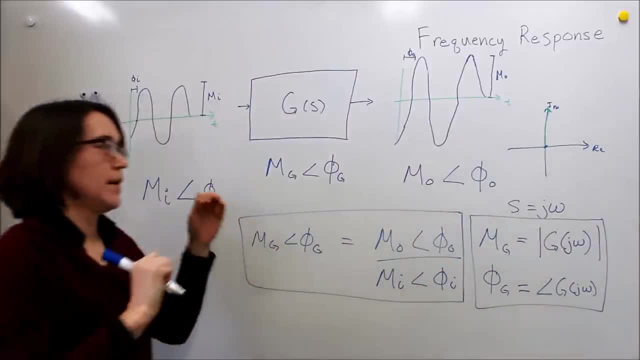 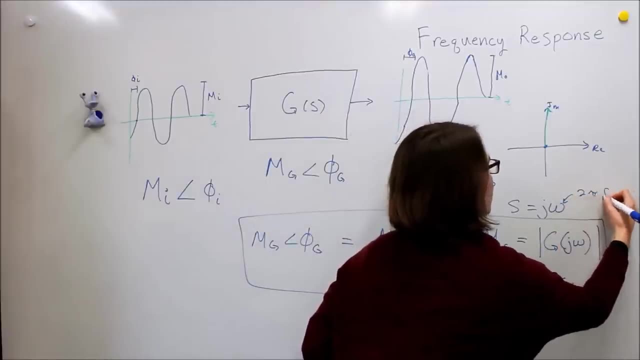 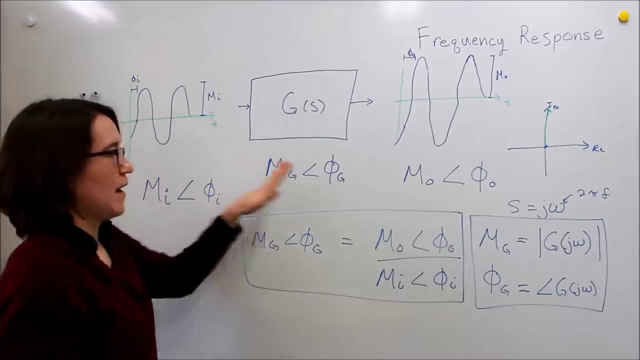 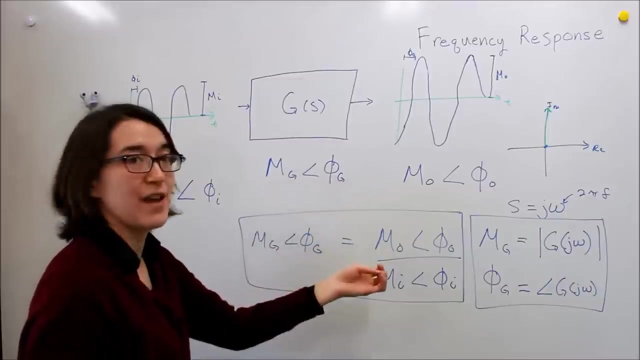 okay. so one more thing is that this Omega, remember, is two pi frequency and this frequency is in Hertz, so you can put in whatever frequency, your input is here and you can figure out how this system will affect, so how the effects on the magnitude and the phase at that given frequency. okay, so we're going to. 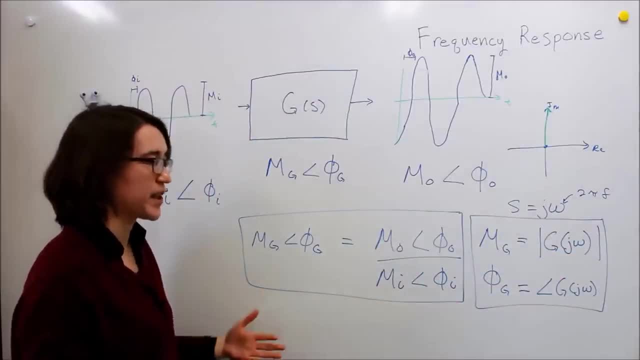 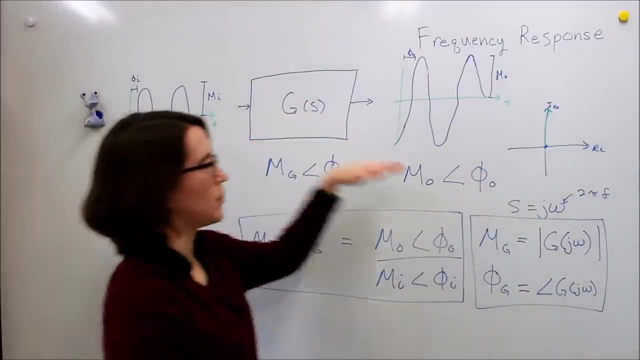 look at how to use this again and you want to be very careful when you are. use this and draw it out in a Bode plot and hopefully that will be a little bit clearer. But to find the frequency response you have to take your actual G of s here you put in